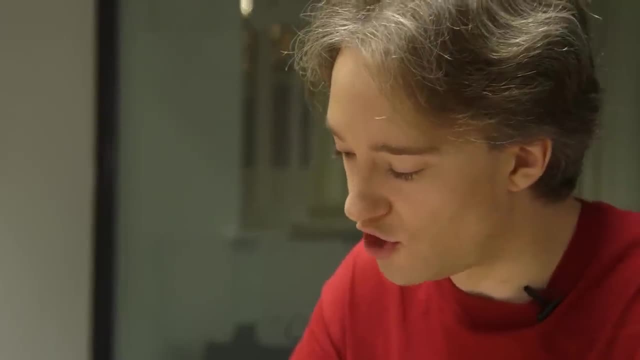 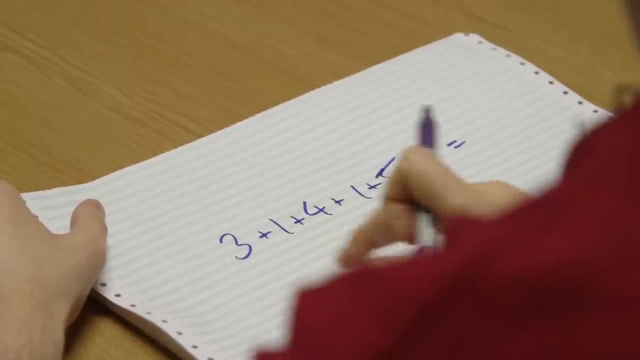 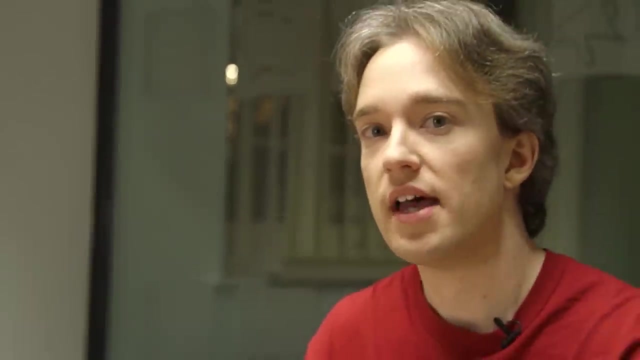 who it says it is. The simplest hash algorithm I can think of would just be something like that: That's five, add up all the digits in the file, which is 4, 9,, 40,, 23.. That's not a good hash algorithm for a few reasons. 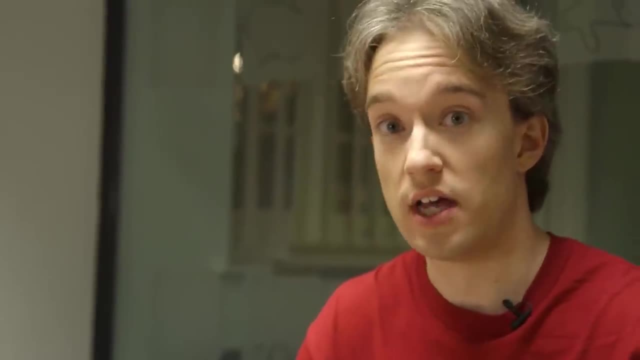 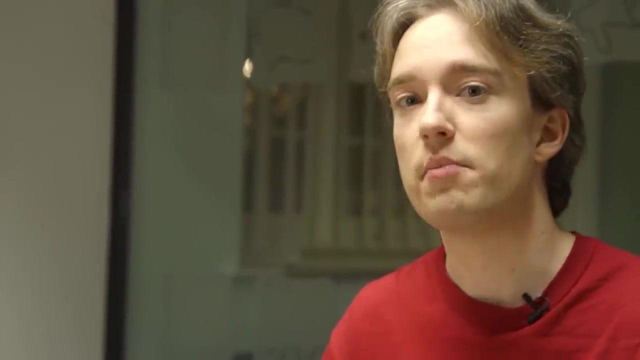 Hash algorithms have three main requirements. The first one is speed. It's got to be reasonably fast. it should be able to churn through a big file in a second or two at most. but it also shouldn't be too quick. If it's too quick it's easy to break, and I'll explain that. 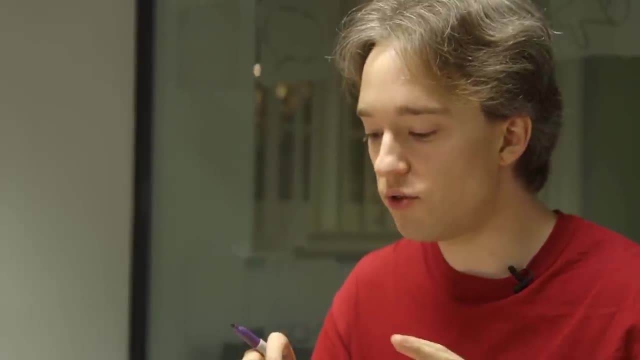 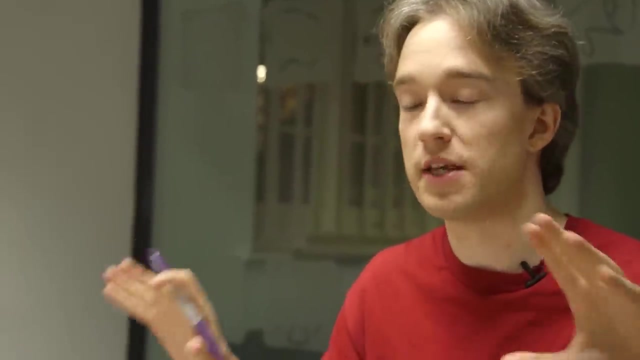 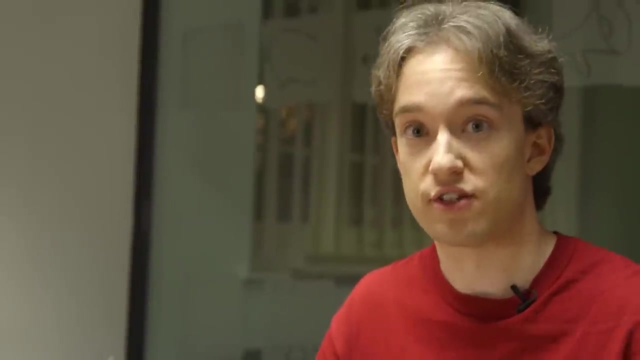 later. The second requirement is that if you change one byte, one bit anywhere in the file- at the start, at the middle, at the end- then the whole hash should be completely different. This is something called the avalanche effect. If you're interested in how this is achieved, do look up the actual algorithms themselves. It'd take me an hour to explain vaguely how they work in a friendly way. but if it's your kind of thing, do look it up. But suffice it to say if one bit gets flipped anywhere in the message, then the whole hash is completely and utterly different. 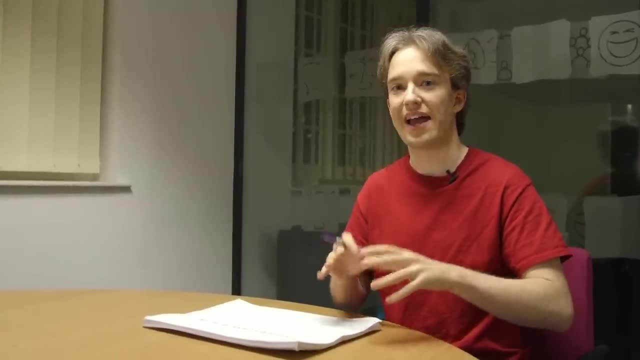 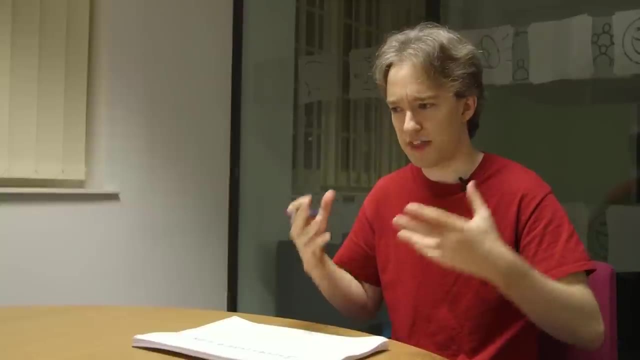 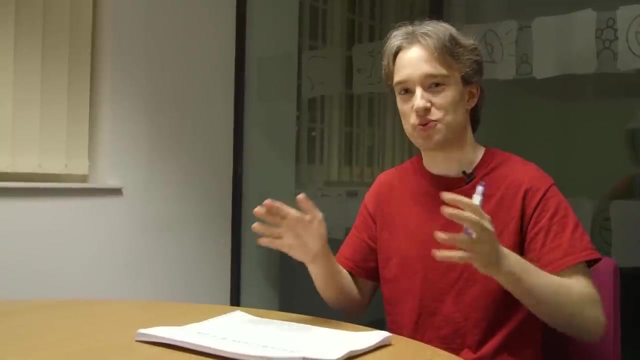 The third requirement is that you've got to be able to avoid what are called hash collisions. This is where you have two documents which have the same hash. Now, obviously, there is a mathematical principle called the pigeonhole principle You have, If you have 50 pigeons and 25 pigeonholes, you have to stuff two pigeons into one of. 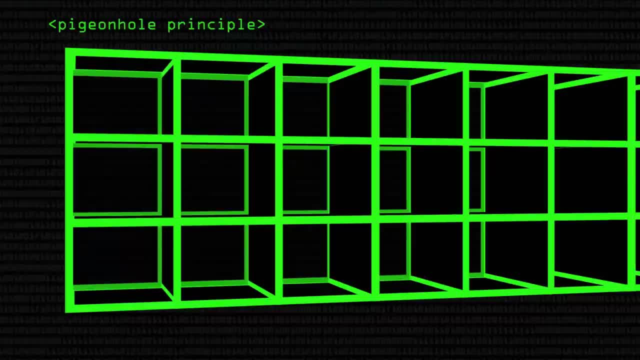 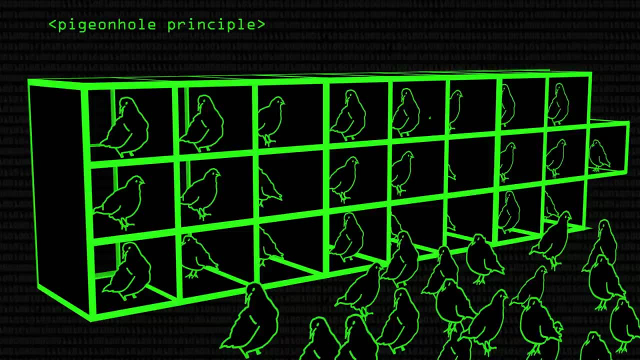 the pigeonholes. That's a terrible analogy when you say it like this, but if I explain it, There are incredible numbers of documents out there. possibly The hash, meanwhile, is just one fairly long number. There will be files out there which naturally have the same hash. And that's OK because the odds against it are so unlikely that we can deal with that. It's never going to happen, naturally. But if you can artificially create a hash collision, if you can say create a file and change a name, then we have a problem. 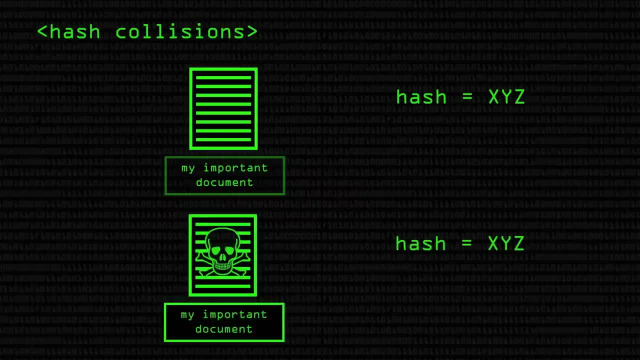 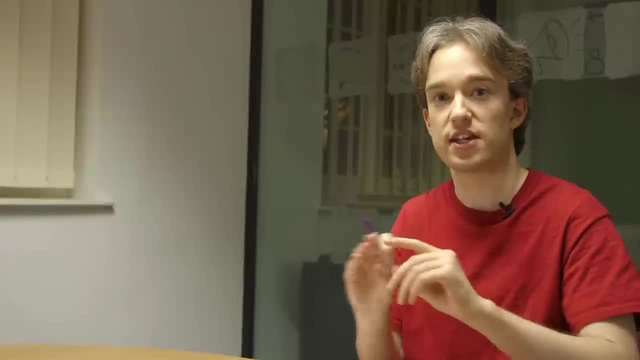 And that's where security comes into these, Because if I can make a file that sums to a certain hash, then I can fake documents. I can send different things and have the signature match. So let's say I have an important document, something that's. 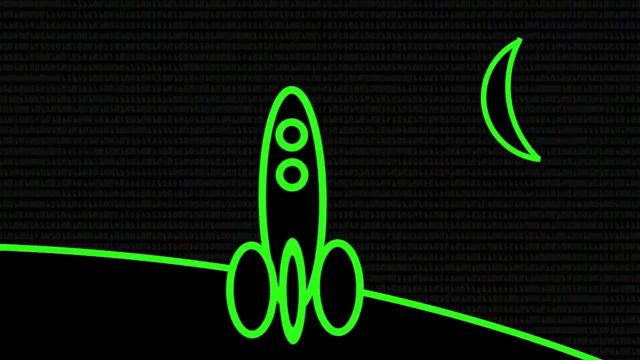 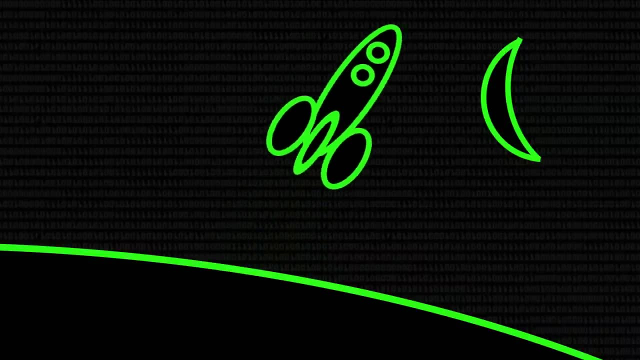 I don't know The permission to go to the moon. I don't know why I said that. Yeah, permission to go to the moon. Let's say that, And it's got someone's name on it And that file is sent. 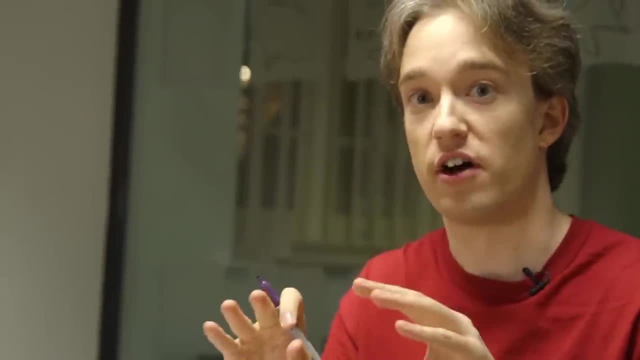 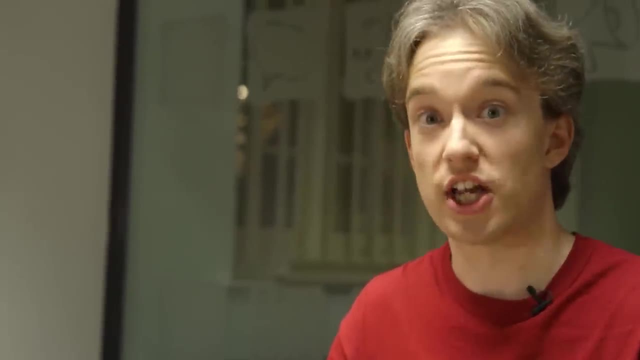 And along with it, Through other channels, comes this hash to verify that this is actually the document. Now let's say I can intercept that file and I can change it, but because the hash algorithm is broken, I can change it. 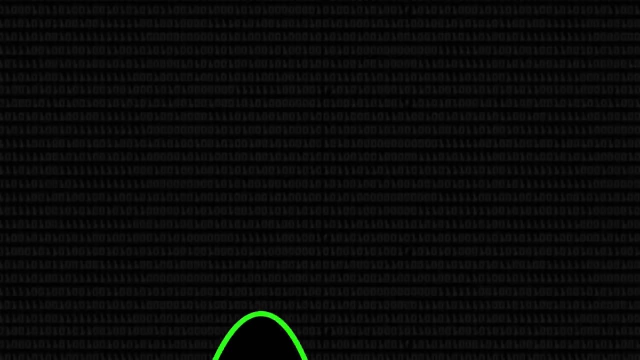 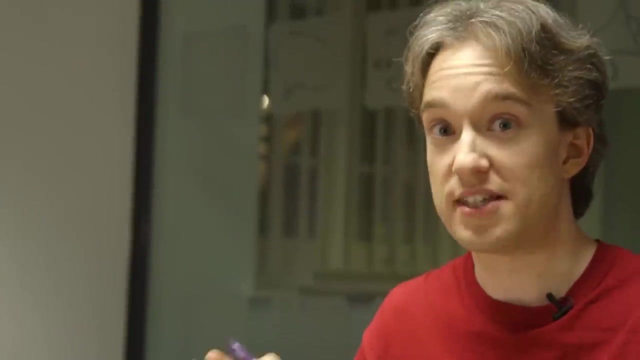 I can change the name, I can change the date, I can change whatever, and I can send someone else to the moon, because I can make this hash the same through carefully tweaking the bytes. Now, it's incredibly difficult to do that. In practice, you'd want a massive file and a lot of computer code, But there are old hash algorithms like MD5, which was used for many, many years, which now have these collisions out in the wild and are considered broken. 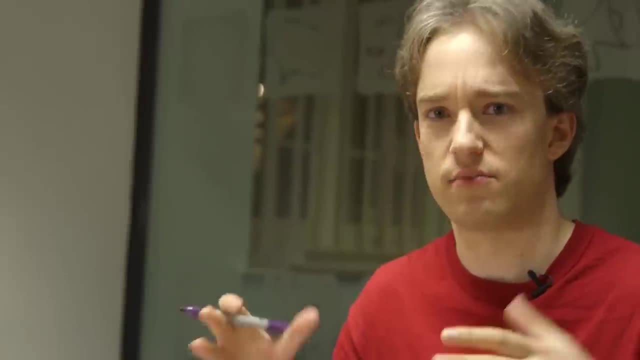 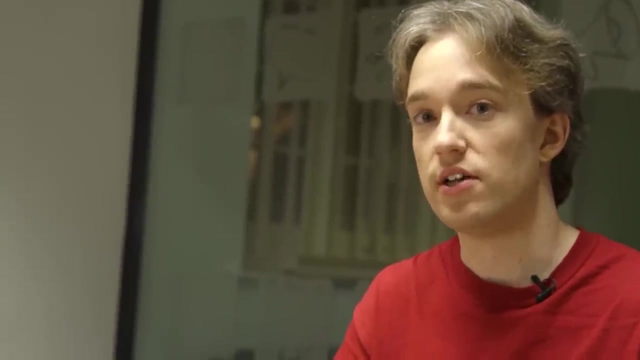 Because you can get a file, not like a document with text in it, but computer code, anything like that, where it's possible to send something malicious and have it come out with the same hash. So this is important. This is where speed comes in. If the hash is too slow, no one will want to use it. But if the hash is too fast, if you can create new ones in a few processes, then you can fairly easily create documents that match a particular hash. It is, in a very real sense, an arms race. As I said, for many years MD5 was the accepted algorithm And it's still used for a few things. But MD5 is now thoroughly broken because computers are fast enough and there are a few interesting tricks you can use to try and create hash collisions deliberately. 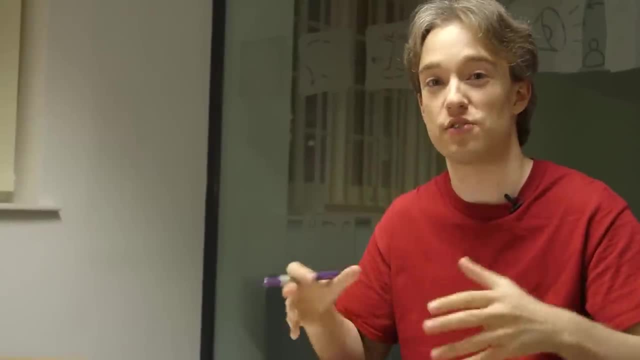 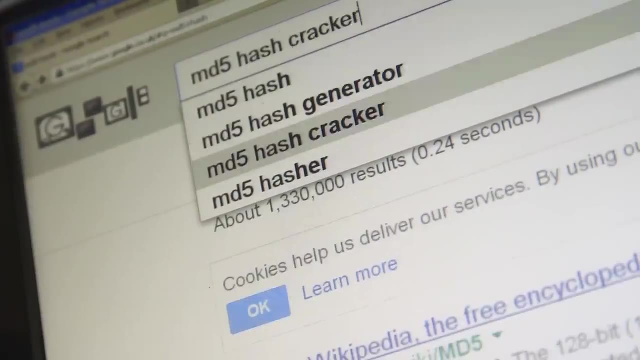 The other problem with MD5, is because it was used so much and it was used everywhere on the web. Google has become an exceptionally good resource for breaking them. You wouldn't want to store a password this way. I'll talk about that in a later video. 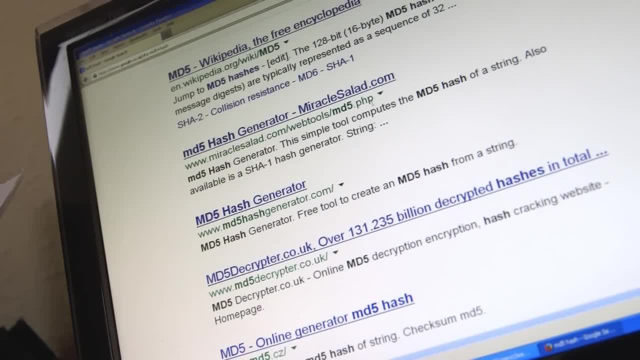 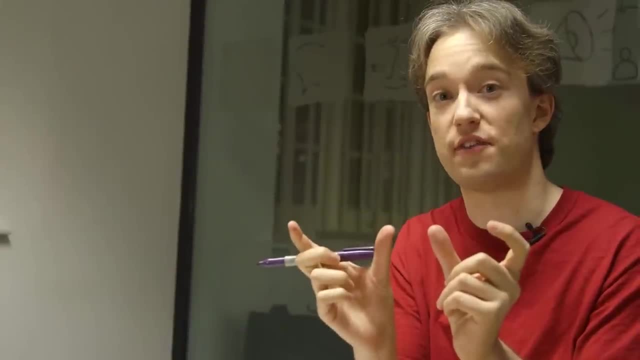 Don't use something like this for storing passwords, But people did For many years people did And in a lot of cases a word will be stored next to its MD5 hash for some reason, If you type an MD5 hash into Google, 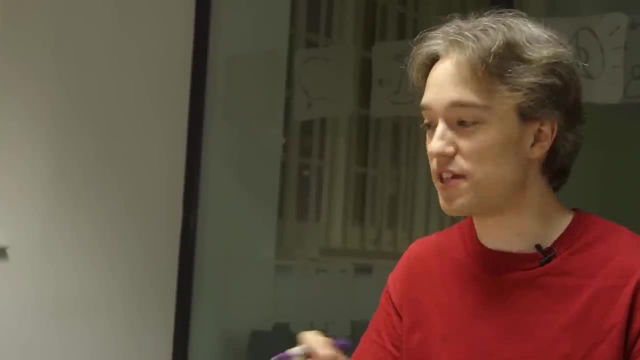 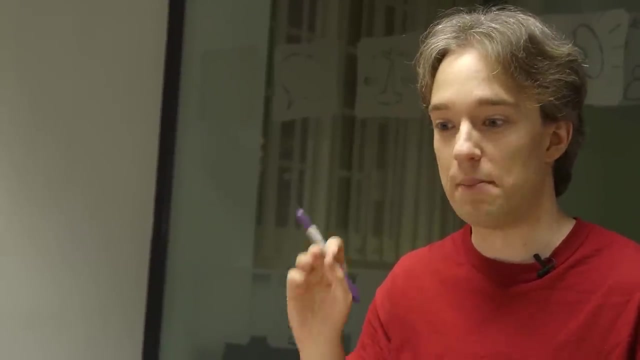 frequently the word it was hashing comes out, Which means that for pretty much every word in the English language and a lot of other passwords besides, the MD5 can be solved by typing it into Google. So MD5 is comprehensively, constantly broken. So everyone moved to something called SHA-1.. And now there are rumours that that might start to be broken soon, if it hasn't already. because computers keep getting faster, Hash collisions are easier to generate, So everyone is moving to SHA-2. 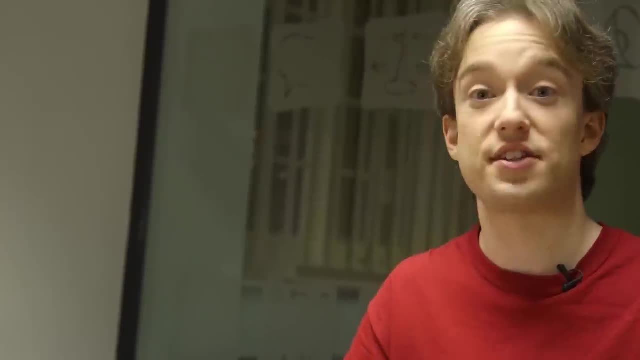 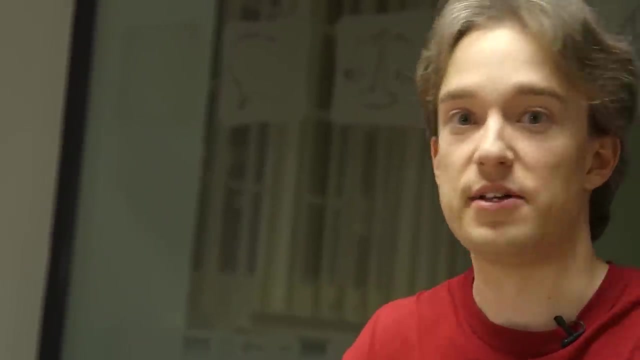 Which, for the time being, is secure. SHA-3 is going through the process of being ratified by all the agencies now, and in a few years that'll be the standard I mean ultimately. I should really emphasise this. 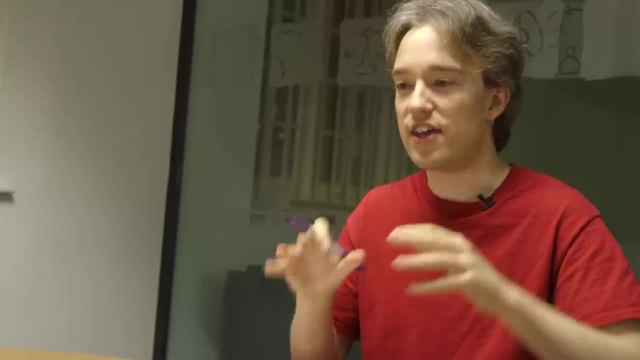 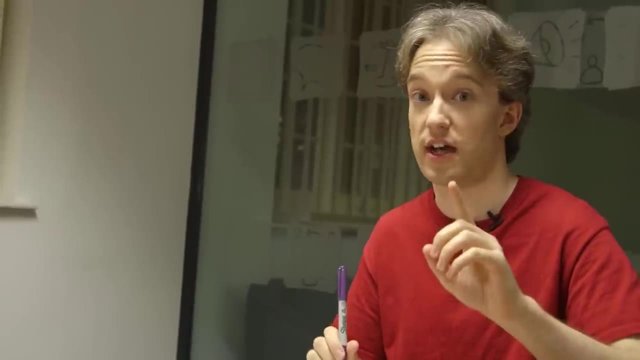 Don't use this for storing passwords. I'll talk about that in a later video. These are used for verifying files, For verifying transmission, And that's all they should be used for. There is one last thing, Which is that occasionally you will see download sites offering software.